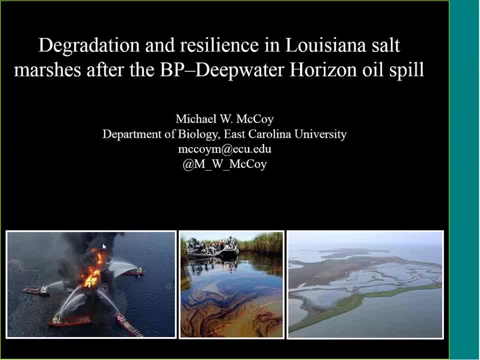 We've both since left Florida and moved independently to North Carolina, Brian to Duke and myself to East Carolina University, But the work was done here while we were both at University of Florida, in the Barataria Bay region of Louisiana. So the work I'm going to tell you about was published in the Proceedings of the National Academy of Sciences. 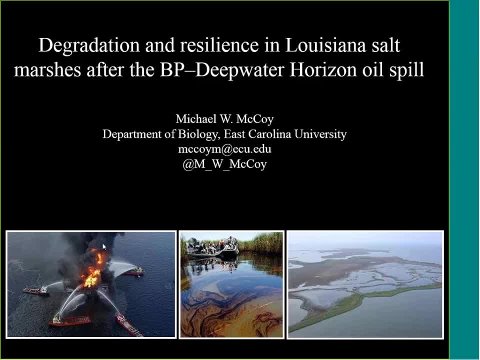 And it's a research story that leaves us with both a message of optimism and concern about salt marshes in response to oil spills. But before I get into the science, I want to introduce you to what salt marshes are, for any of you who may not be familiar with them. 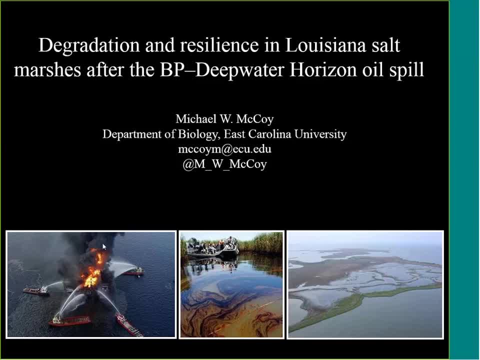 I'll tell you a little bit about why they're important for us And I'll tell you a little bit about their ecology- natural ecology- and then about the effects of oil spills. So salt marshes are one of the most common coastal habitats along the western Atlantic coast, as well as the Gulf Coast. 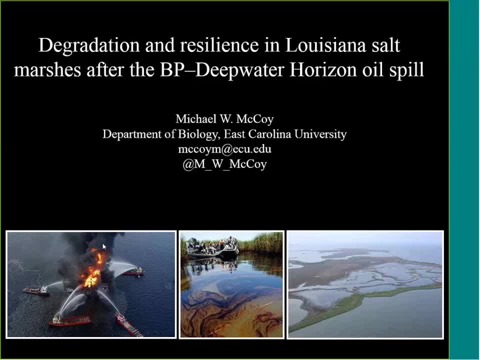 They consist predominantly of salt marshes. Salt marshes are one of the most common coastal habitats along the western Atlantic coast, as well as the Gulf Coast. They consist predominantly of a single species of plant: Spartina alterniflora. There are a few other species, but they're really low diverse systems dominated by Spartina alterniflora. 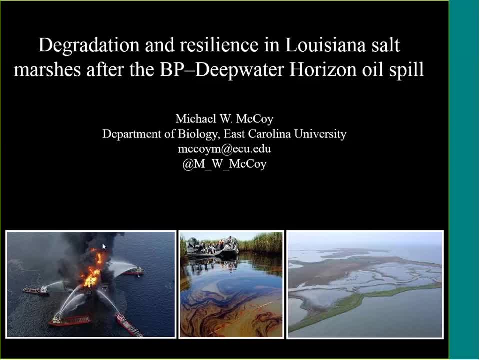 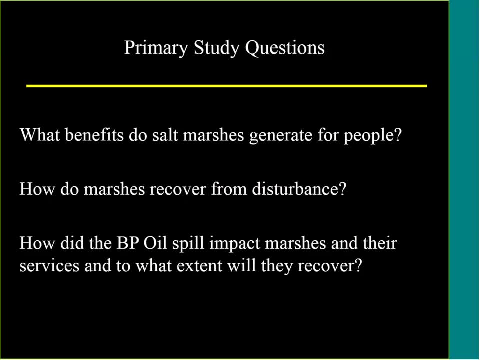 And you can see them, you know very commonly as you go over bridges and stuff along the east coast, And they're very important for a variety of reasons. So as I go through this, just to give you a little bit of a road map, first I'm going to talk about what salt marshes do for people. 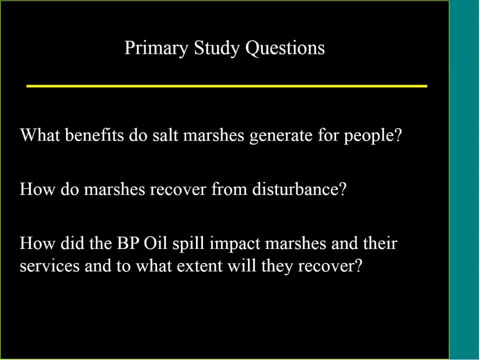 Why are they valuable? Why do we care about them so much? And then I'll talk about how they recover from natural patterns of disturbance which they have- a variety of things that cause disturbances in salt marshes that they must recover from. And then I'll finish off by talking about the work that we did, actually evaluating the effects of the Deepwater Horizon oil spill on salt marshes. 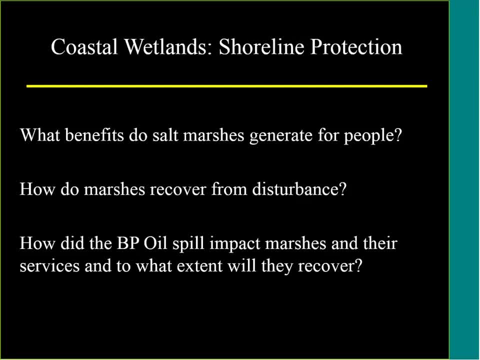 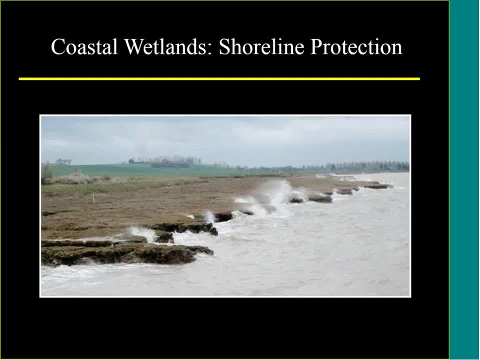 and how they're recovering from those effects. So one of the primary things that we gain from having coastal salt marshes intact is coastal shoreline protection. So having our borders along the edges of bays and oceans buffered by these salt marshes actually reduces wave energy and wave action. 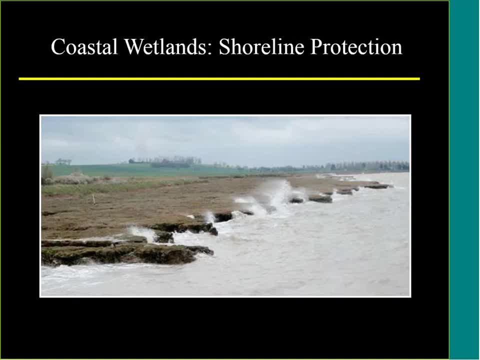 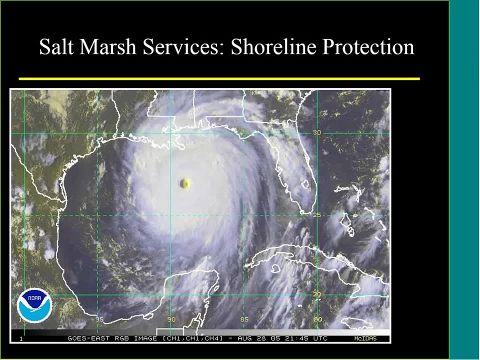 and it slows the flow of water inland, such as from storm surges during hurricane events, etc. Just as an example of that shoreline service. I'll bring up this picture, since it's relevant to the area that we're talking about, where the spill occurs. 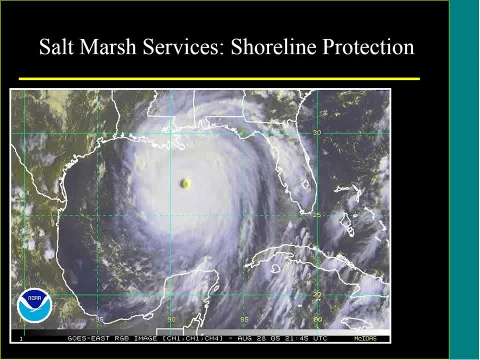 And this is Hurricane Katrina, which, as we all know, was a devastating storm, largely because of the impacts of the storm surge. Now, while salt marshes likely couldn't have stopped this magnitude of devastation, they likely, having more intact salt marshes, could have reduced the effects. 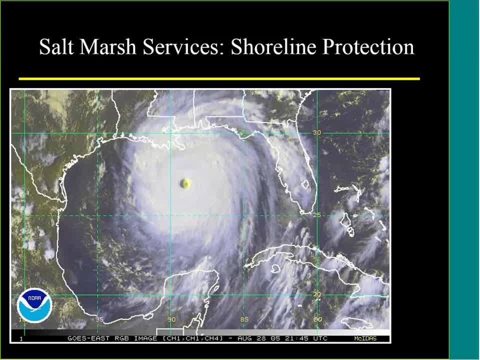 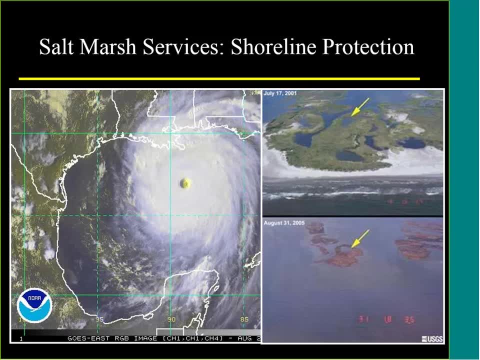 and maybe stopped the effects of less severe events. So it's been suggested that per mile of continuous wetlands along the coast can actually reduce the size of storm surges by as much as 8 inches. So if we think about the storm surge coming in here, we can see here: 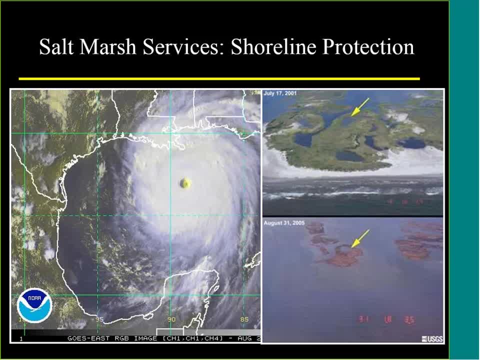 in 2001,. this is an area along the coast of Louisiana, here with intact marshes which, by about five days post-Katrina you can see, is much less extensive, And so we lose several inches of salt marsh, which results in potentially a couple of feet of reduction of storm surge. 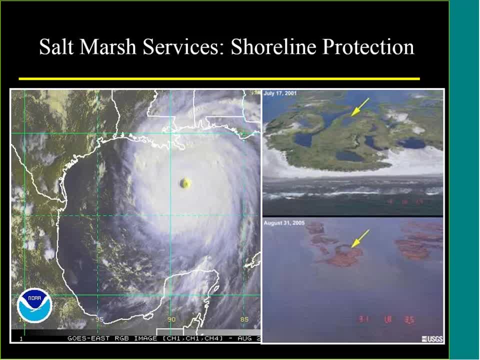 just by natural degradation of this system. In this case, the loss of salt marshes along this region is largely driven by changes to the flow regimes and other sort of anthropogenic disturbances upstream, But regardless we're losing salt marsh and that has significant, large impacts. 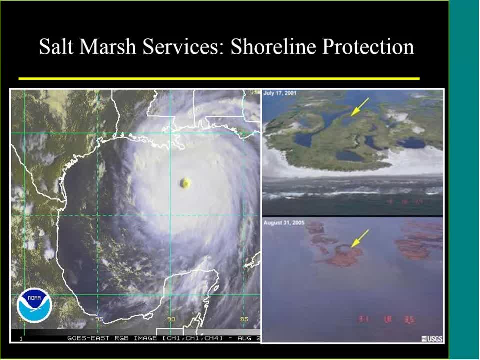 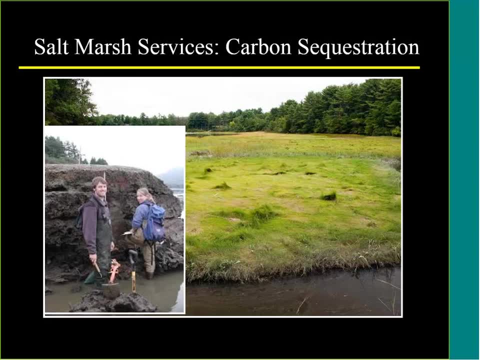 on how systems respond to large coastal events. Another important service of coastal salt marshes is carbon sequestration. These are incredibly productive systems. despite the fact that they have only a low diversity of plant species, They sequester a lot of carbon from the atmosphere. 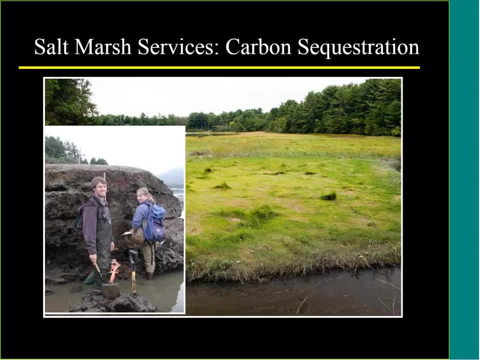 There's a high plant growth during the growing season. That plant growth takes the carbon out of the atmosphere, turns it into biomass, which then is deposited into soils, which accumulates for thousands or tens of thousands of years, and that carbon stays bound up in the soils in these marshes and not released back into the atmosphere. 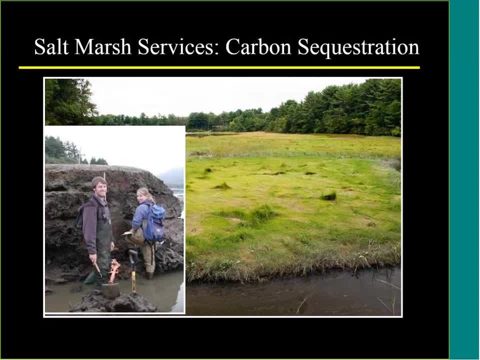 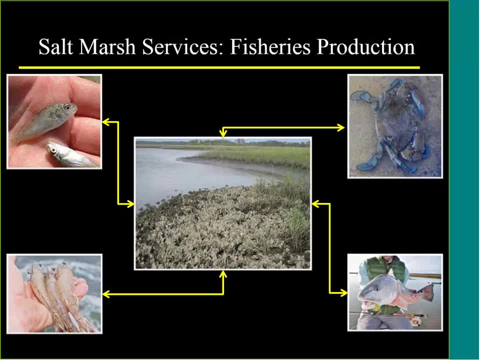 So we have this really important service of carbon sequestration- carbon sinks, as a matter of fact. So A service of these systems that most people are probably more familiar with is their role in production of fisheries and tourism, For example, along the Gulf Coast. these systems are associated with more than $10 billion of revenue. 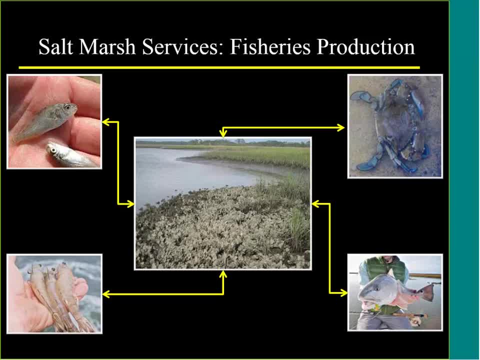 in the source of fisheries and tourist activities, because they serve as nursery grounds for juvenile fish, especially those fish that are commercially important for shellfish, like shrimp and crabs- Blue crabs use these habitats for foraging. They also serve as foraging grounds during high tide events for other, more large fish. 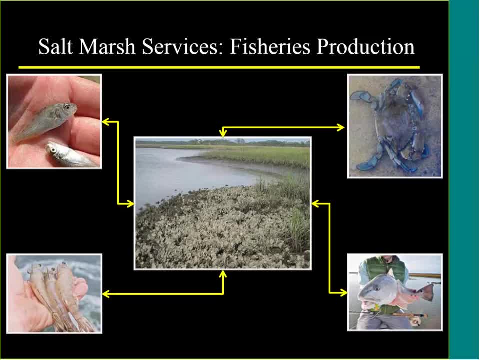 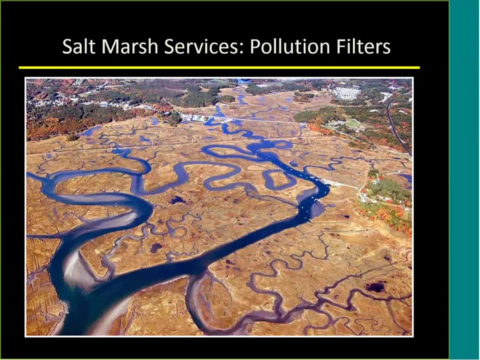 that we may be interested in, for example, for game fishing. So we also have also a huge component of shellfish. These systems are incredibly financially valuable for a variety of reasons, And the last service- I'll talk about things that these things give us. 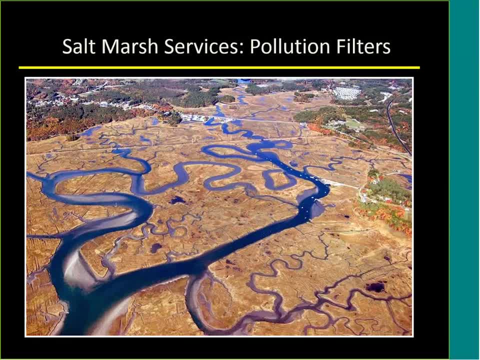 is Spartina alterniflora, even more so than other marsh plants, are able to sequester pollution from water, So they serve as these buffers along the coast, for I talked about incoming waters in terms of storm surge- but they also take contaminants out of water that's flowing back out towards the oceans or to the sea. 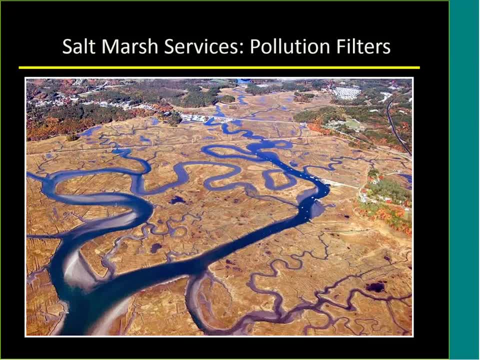 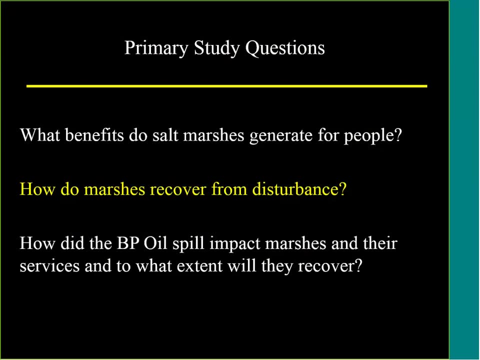 So they have this capacity to buffer both taking out nitrogen as well as things like pesticides and other contaminants from the water before it moves out into our coastal systems and affects things like fisheries Pollution filter. filtration is another important service, So that just gives you a general idea that these systems are quite important. 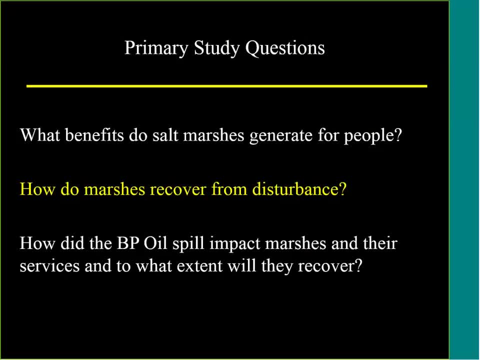 beyond just that. they're really attractive and they smell like sulfur, But they actually provide a variety of services. So next I want to talk about what are the causes of disturbances in these systems and how do they recover from them naturally, And then we can talk about how they recover from a large antigenic disturbance like a oil spill. 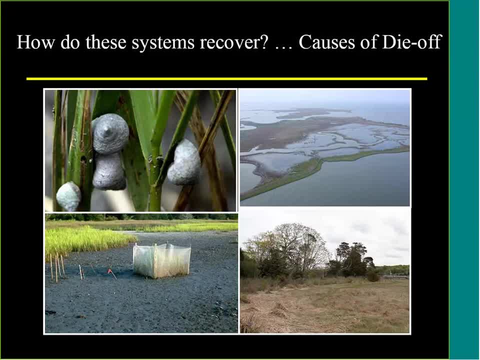 So salt marshes have been experiencing, especially along the western Atlantic, have been experiencing massive die-offs for many decades now And that's been the subject of an intense debate and a lot of research And it's been attributed to a variety of causes. 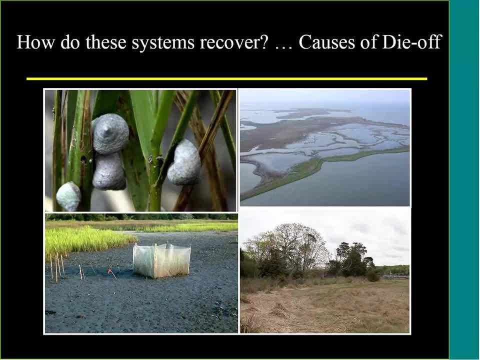 One of those is increased drought events, which increases the salinity of the soil, which can kill off plants and leave these massive mud-flat areas where the spartina is completely missing. It increases erosion rates and other processes that further damage the soil. 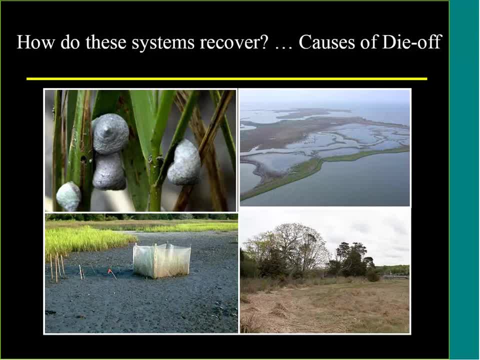 In other locations they've been attributed to drowning. Basically, you get too wet of conditions, which actually ends up causing rottens in the roots, because they depend on a tidal cycle where they dry and they become inundated periodically. But if they stay inundated too long, it's actually not good for them. 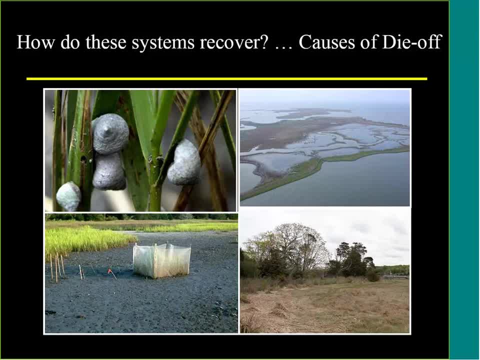 And there also have been suggested that they're dying off as a result of top-down forces. So, for example, if you look at the ocean, you can see that the salt marshes grow because of consumers that are foraging on these things, down to the point where they're converting these grass systems into mud-flats. 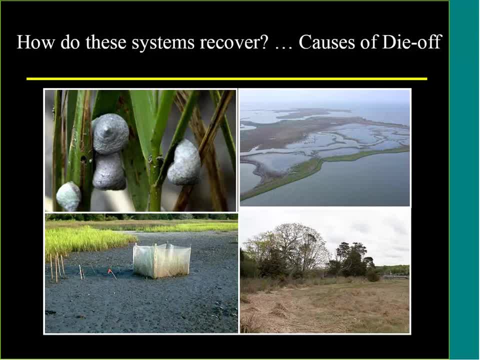 And that's been driven primarily by this very common snail that lives in these salt marshes. It's called a periwinkle marsh periwinkle snail, And the snail itself doesn't actually eat the spartina. It creates little radular gashes in the stems where a fungus grows. 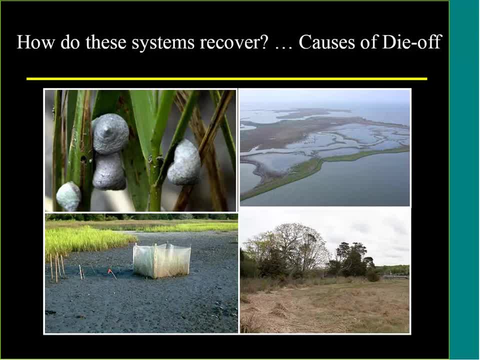 and the snail goes back and eats the fungus And you get these massive feedback loops where the density of the snails increase to a point where they cause the plants to die through the process of forming this fungus that's consuming it. So in some locations you have these top-down forces. 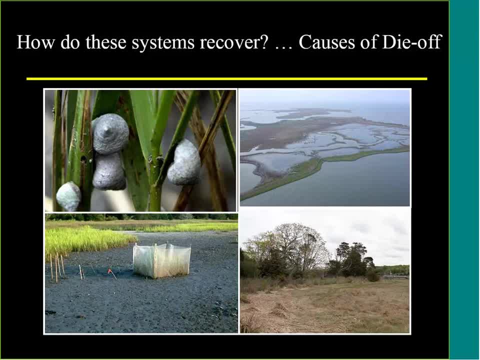 consumers or introduced consumers, like ungulates, causing die-offs In other systems. you have these sort of bottom-up processes, But in reality in most systems you probably have all of these things sort of working in concert, And so we do have die-offs that are a concern. 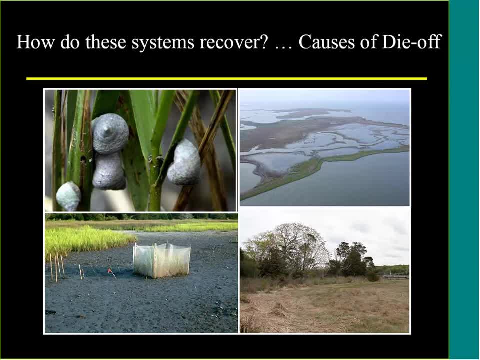 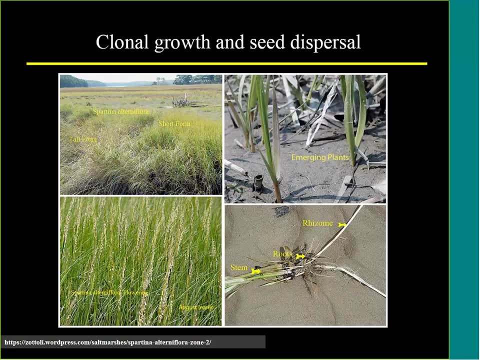 But these systems also tend to be quite resilient, And so they can actually refill these areas that have die-offs through a variety of processes, That's being seed dispersal one, because, like other plants, these spartina- here you can see- produce flowers and seeds. 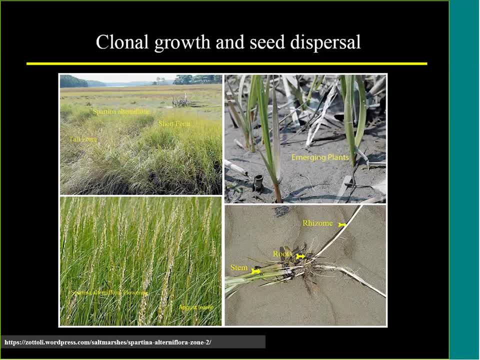 and these seeds are deposited on the marsh surface to germinate and recruit as new plants. But more commonly these die-off areas are recovered via clonal growth. So these plants produce these thick matrices of roots under the soil, so this underground biomass. 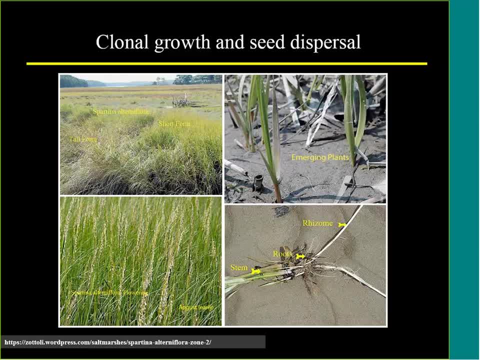 And plant growth is more important than the above-ground plants for maintaining the stability and the structure of these salt-borne systems, And so one of the things they do is you have this die-off event occur and they produce these long rhizomes which spread out into the now defoliated area. 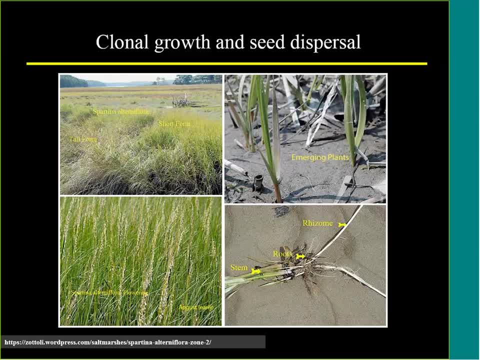 and produce new little plants, as you can see here, these emerging plants, And so this clonal propagation is one of the primary mechanisms that these sort of die-off areas actually produce. They're used to recover And, as a result of that, the rate of recovery of these systems. 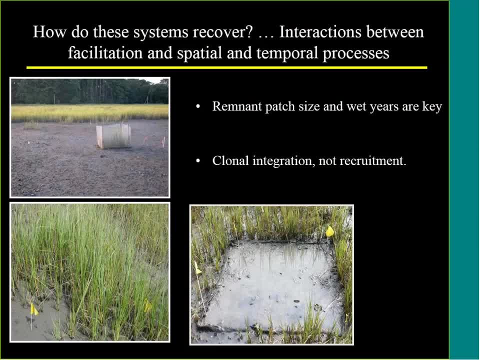 is driven both by the size of the die-off area, so the size of the bud flat and the sizes of the remnant patches that are in those die-off areas. If they're clonally growing outwards from some little reservoir plant that's left in the middle, then the size of that little patch remnant 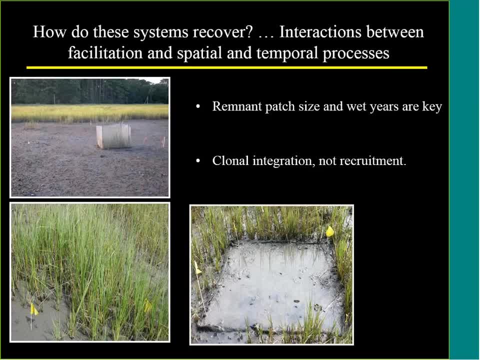 is going to determine the rate at which it's recovered. So we have to think about that when we're thinking about managing as far-time regrowth areas- And you can see that it's actually predominantly clonal integration here, because this is an experiment that Dr Silliman did- 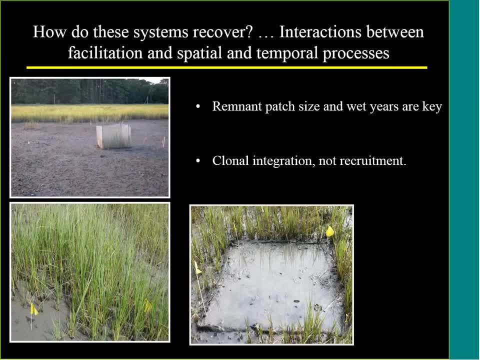 where in some cases it blocked off, it buried a barrier to the clonal growth and in other cases left the bud flat, unburied, without barriers. And you can see where the barrier was Preventing clonal integration, you actually got no plant growth. 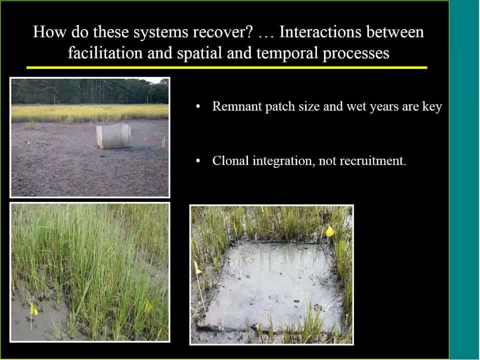 So it suggests that there's clonal integration. at least in this case, that's more important than seed recruitment for covering the system. That's also really important because clonal growth actually comes with an already pre-established root matrix, which is actually really important for reducing erosion. 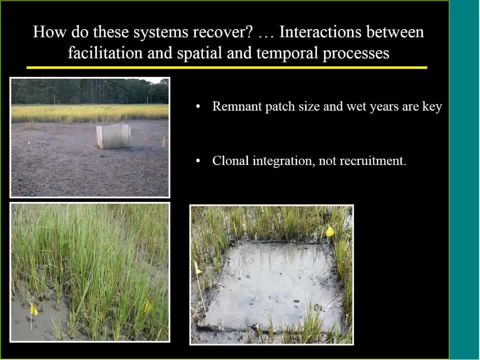 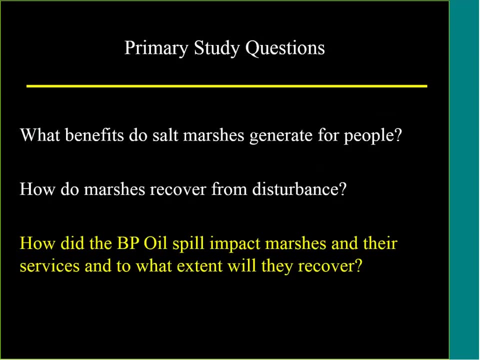 So systems are vulnerable to a variety of stressors, but they actually are quite resilient and regrow quite rapidly to some die-off situations because of this clonal regeneration. So that gets us to the actual reason that you invited me here, and that's to talk about how the DC Deepwater Horizon oil spill. 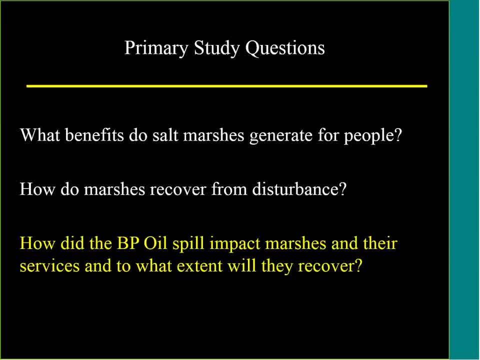 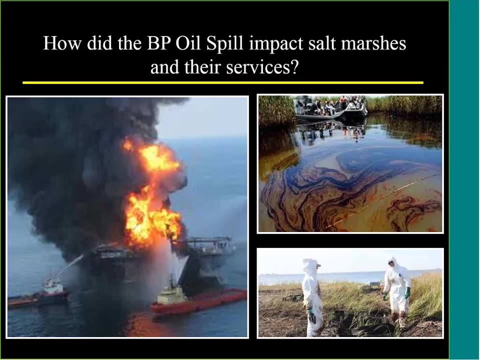 impacted marshes, the ecosystem services they provide, and to what extent can we expect them to recover from these kinds of large-scale impacts? So, as we all know, in 2010, we had this massive event that resulted in the movement of oil onto the shoreline. 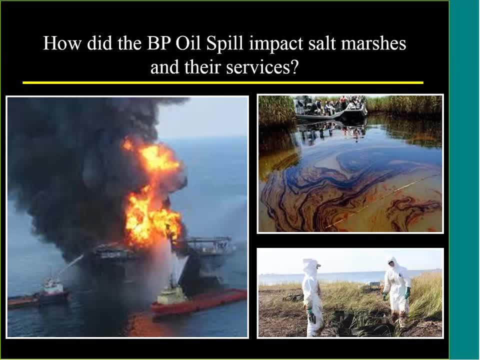 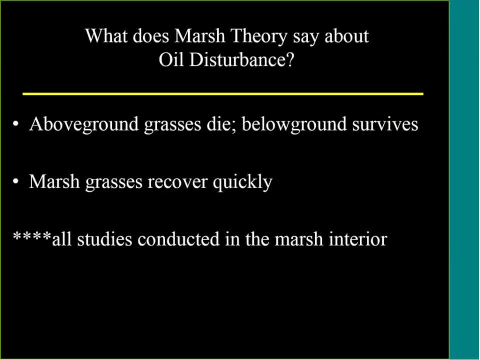 and it caused a variety of problems And we went into this study to look at the effects of this oil on the marsh grasses, with a great deal of work already in place that we could sort of use as a starting point for thinking about how these marsh grasses were going to respond. 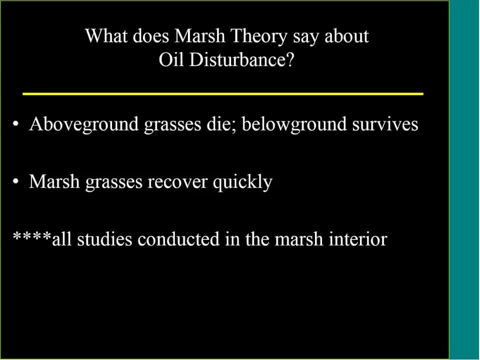 And we knew that. put oil on the leaves of these grasses, they tend to die. But most of the work suggested that had been done out there- and there was a fair bit of it- suggested that the below-ground root matrix stayed in place. 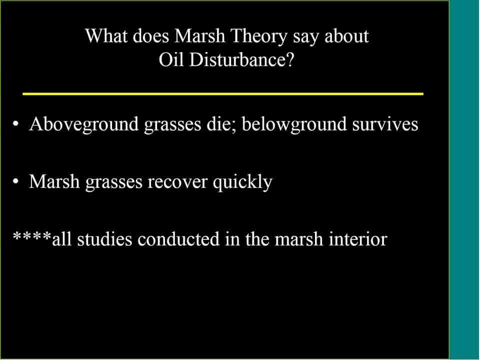 And as a result, you got this really quick recovery of the marshes even after an oiling event. This was really encouraging because what we were hoping is that we would see this mass really rapid recovery after the initial oil coverage. But we also recognized that almost all of the studies 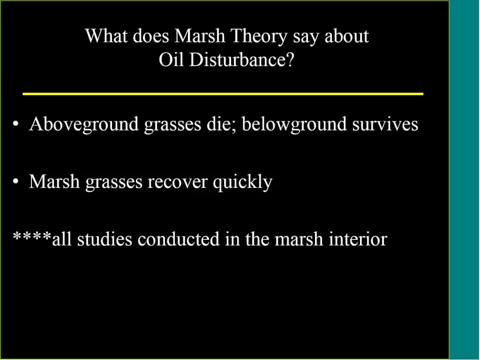 that had been done up to this point were done on plants that were in the interior of the marsh, far from the edges of the marsh, Far from the water. So we were concerned that maybe some of these studies ignored this really important factor, and that is that these really marginal marshes 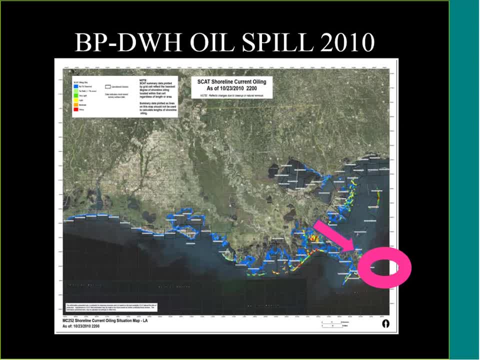 ones that are right on the edge of the water have to deal with additional stressors. So one of the reasons that this was a concern is because most of the impact of the oil, as we've already seen, was concentrated right on the edge of the coast. 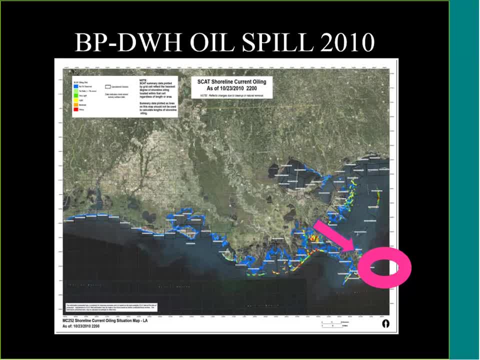 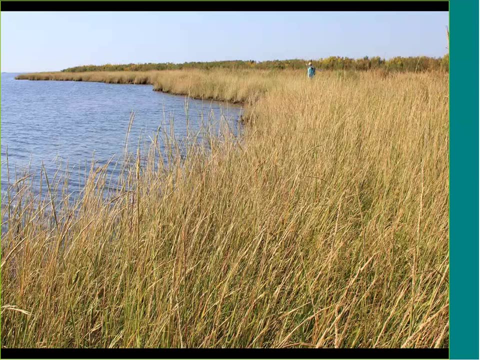 And in fact it was estimated in Louisiana that I think it was more than 75 linear kilometers of shoreline experienced moderate to heavy oiling. So this is really concentrated right on the edge of the water and for great distances. So one of the things that we were concerned- 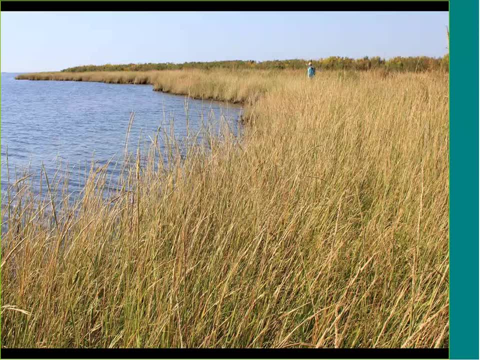 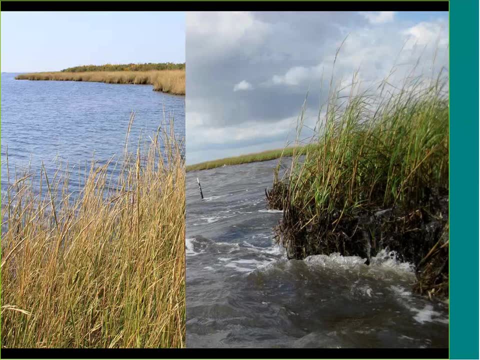 that these systems were dealing with is, if you look at a salt marsh border like this, in addition to dealing with the oil, these guys experienced heavy wave action and other biophysical stressors that might change the impacts of the oil, And so we're trying to get the oil on this system. 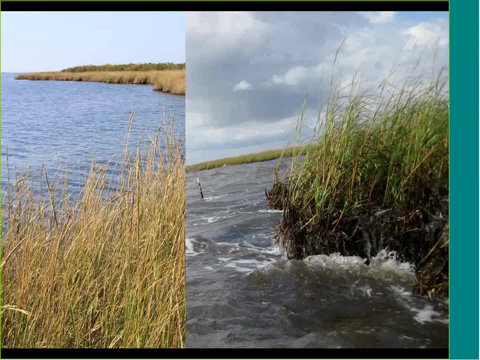 in a way that's not represented by those studies that were focused on the interior grass, And we can also see that many salt marsh systems are already degraded. You can see here this very steep edge on the edge of the salt marsh, which enhances or increases the impact of wave action. 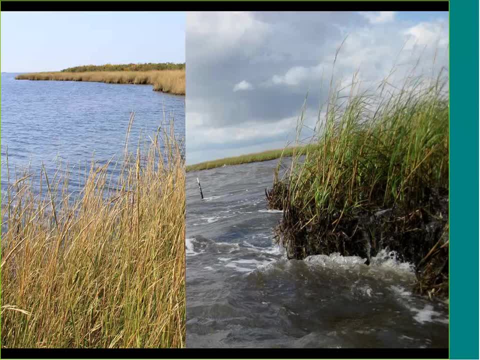 on the earth, especially in the absence of the root matrix. We're really interested in how this biophysical effect of wave action might interact with the oil, And so here we can see that in a similar region of marsh after the oiling event. 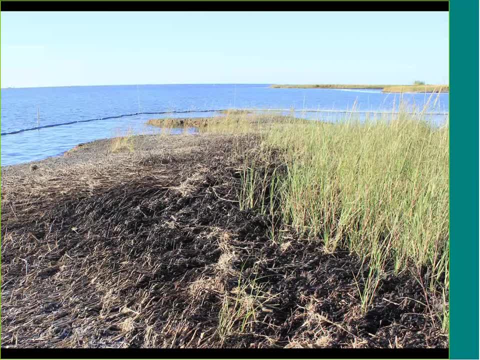 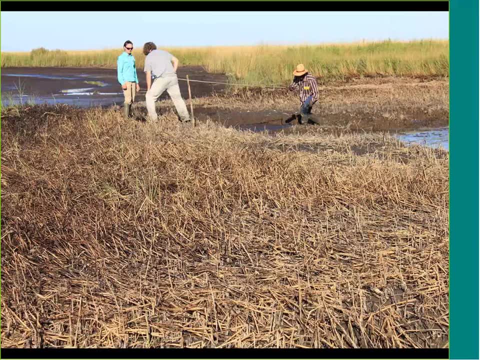 you can see there was a lot of plant die-offs, but it's really concentrated on really along the very edge of the coastline. So what we did is we went out and we set up a series of field surveys, took a lot of field observations. 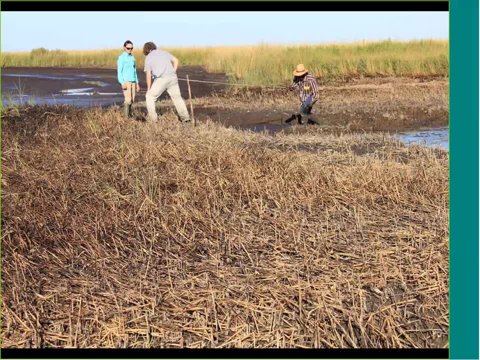 and ran a series of experiments and analyses on these areas to sort of characterize the impact of the oil on the earth. What role did it play on the system? What role did the grass play in either exacerbating or inhibiting that oil impact And then sort of what the response is. 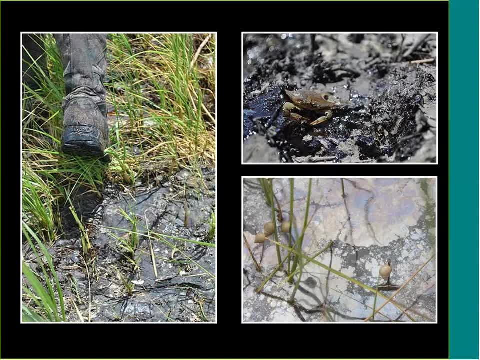 after the impact occurred. And so just to give you a sense of the kinds of data that were collected while doing this study is just: we recorded data on the proportion of the area: total area, not plants or soil-specific, just coverage, area of oil. 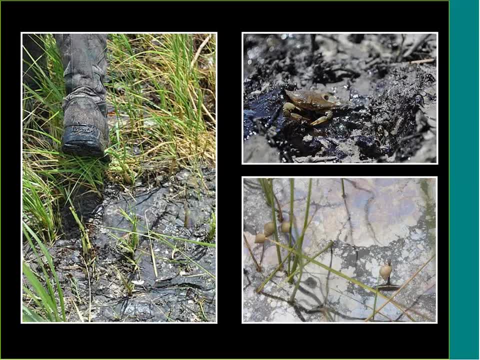 And we did this as a function of how far we were away from the water's edge. We recorded data on the animal life survival of things like snails, crabs, mussels, things that have these systems, And also the amount of oil that was actually. 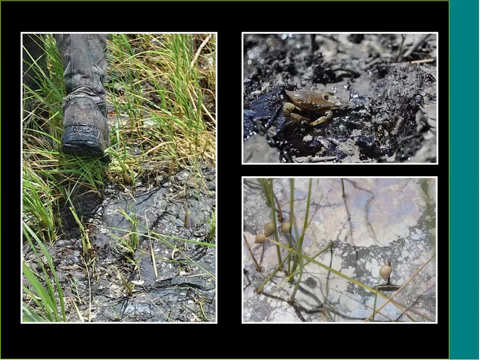 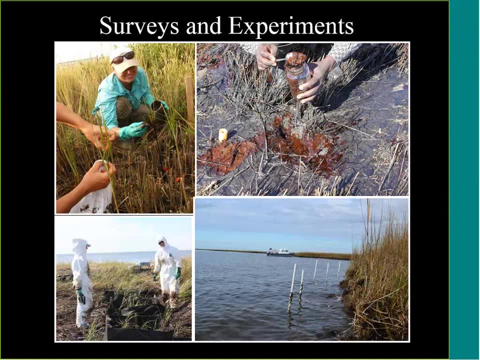 in the plants themselves And survival. of course, We also collected soil sediments to do things like measure polyaromatic hydrocarbons, which is a good tool as an indicator of oil contamination. We did some experimental manipulations and cleaning of plant stems. 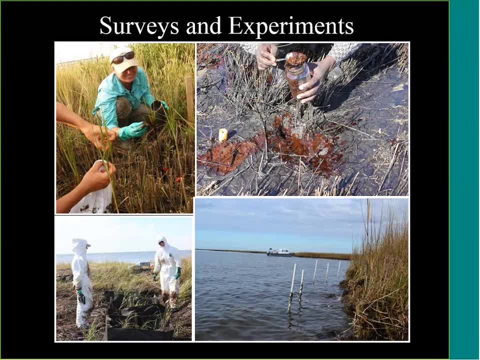 that had been affected by oil. We did oil additions as well as oil removals to sort of assess the effects of the oil on the plants, And we also did some studies to look at erosion rates. So essentially we went out where the edge of the marsh existed. 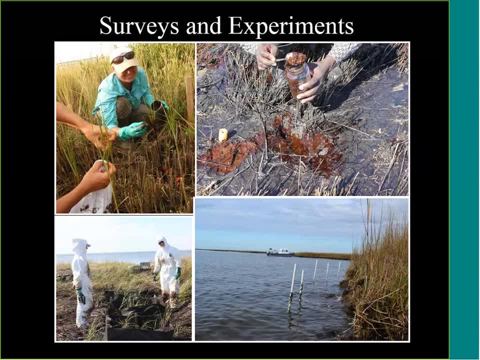 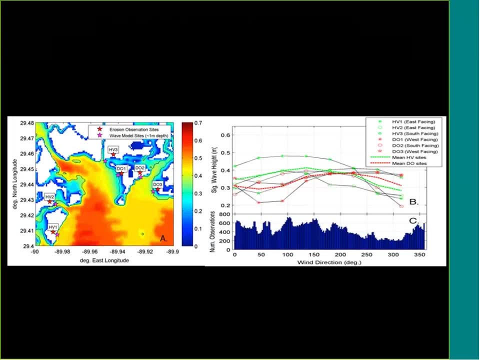 inserted these PVC pipes and then went back and measured them over time to see if the free oiling And so on. this figure here, what I'm showing you, is just a map showing you the distribution of the field sites that we focused on. 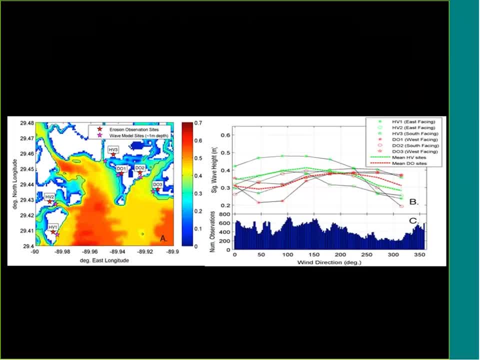 In this case, you can see that the orange stars here are sites where we observed erosion, or actually all the stars are. And the ones that say DO next to them, which is this one, this one, that one, and then the ones that say HB. 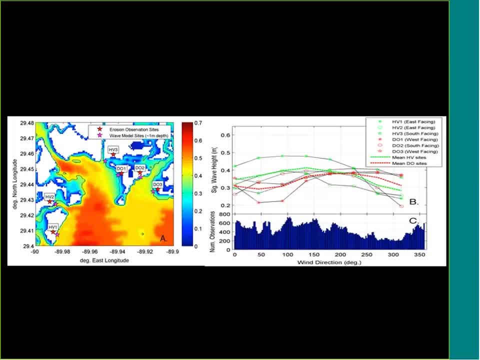 the DO ones are die-off, So these are ones that we suspected to have had a die-off event as a result of oil, And these other ones are the healthy sites that we compared to our reference sites And what this particular analysis here is showing you. 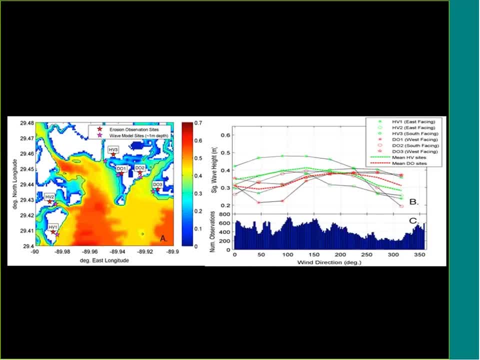 this is a bathymetry model that we used in a modeling framework called SWAN, which is basically a way of using wind action, fetch and a variety of other parameters to estimate wave action in these areas, And what we wanted to make sure of is that our sites. 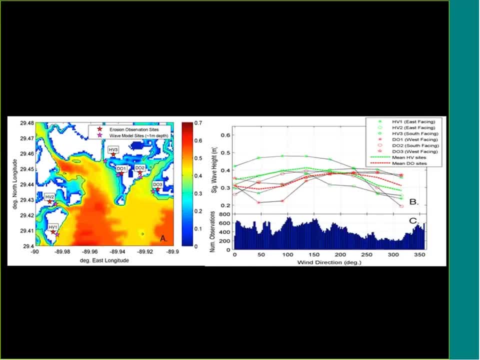 that we were using where oiling had occurred versus our reference sites didn't have different baseline characteristics, could lead to differences in erosion rates or other characteristics, And what you can see is what's showing over here if you focus on this sort of dotted green line. 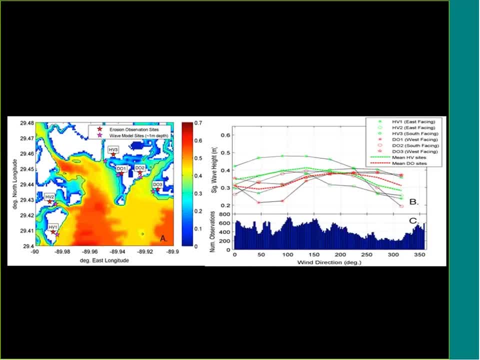 versus this dotted red line is that there are very few differences in the actual wave action experienced by our die-off sites and our healthy sites And in fact, if anything, the healthy sites experience slightly higher wave action than the die-off sites. So this suggests that our sites were pretty well distributed. 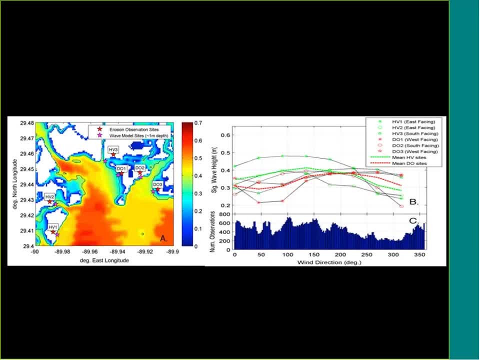 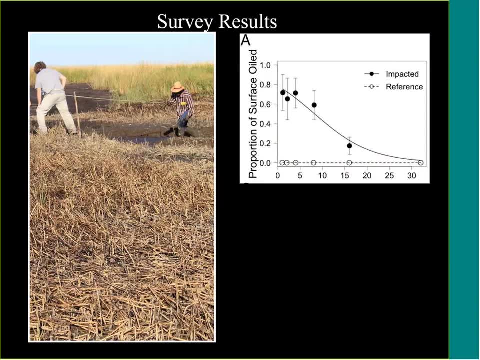 and experiencing similar kinds of biophysical stressors. So then, at each of these sites, we went out and we at different distances from the edge of the water. this isn't actually the edge of the water, but I think it's the best picture I had. 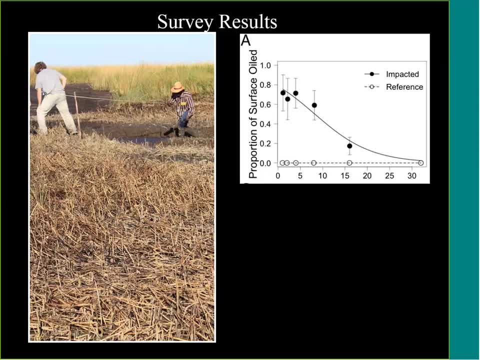 we took data on the proportion of the surface oil, as I mentioned a moment ago, And what you can see here, and we'll show you lots of graphs like this, so I'll just walk you through it so you can get familiar with it. 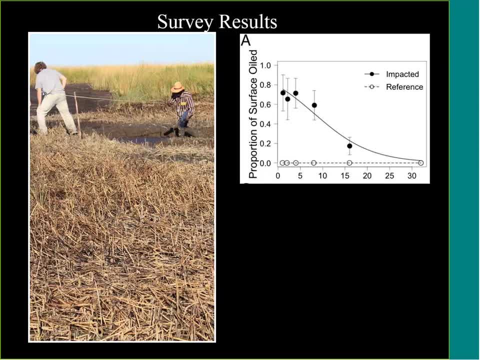 on the x-axis. here we have distance from shoreline, so 0 to 30 meters from the shoreline. The open circles are the reference sites and the filled circles are our impacted sites or sites where oiling had occurred. And this is just to show you the distribution of oil. 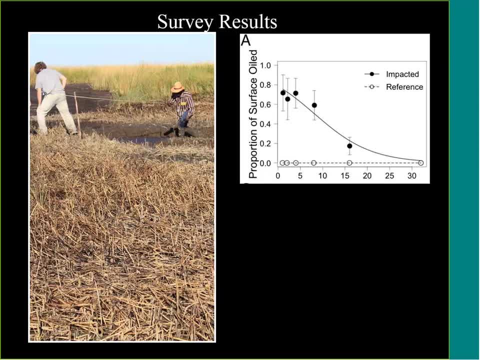 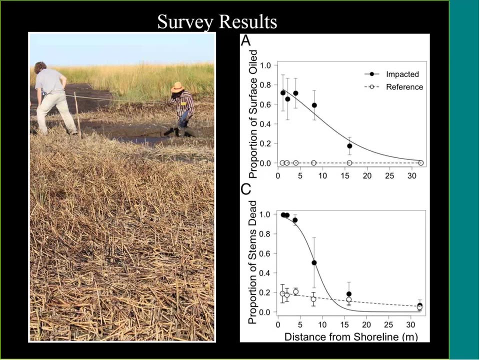 as we moved inland from the edge of the water here at 0 to far into the upper marsh, You can see most of the oil was concentrated really close to the water, as we showed you in that photo, And this is just showing that, in addition to the oil, 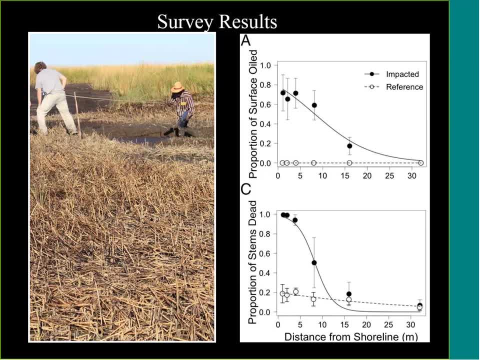 being concentrated near the shoreline. we also see that plants, so this is the proportions of stems that were dead, of plant stems that were dead, again as a function of distance from shoreline, were also much greater, almost all of them right at the edge of the shore. 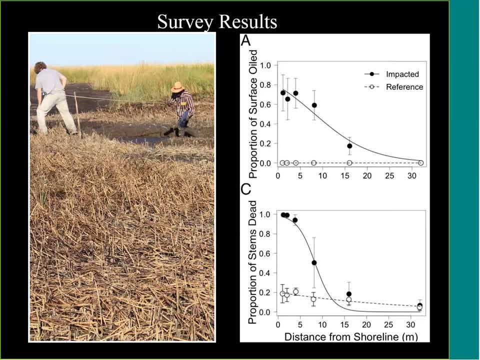 But at about 10 to 15 meters out we start to see high survival again and not different from the reference site. So really really suggest that the impacts of the oil was really concentrated right on the edge of the marsh And this was due in part to the fact that these marshes 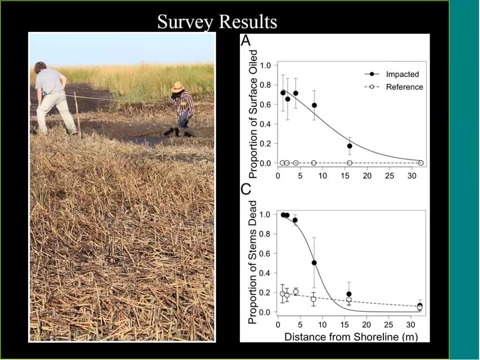 in addition to slowing the flow of storm surges actually also slowed the flow of oil surges, So they actually worked as a boom and restricted the movement of the oil so that it didn't move far inland. It actually remained right at the edge of the marsh. 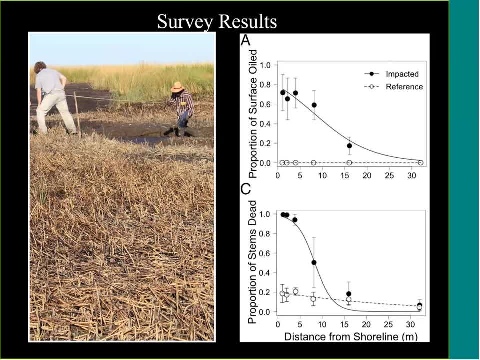 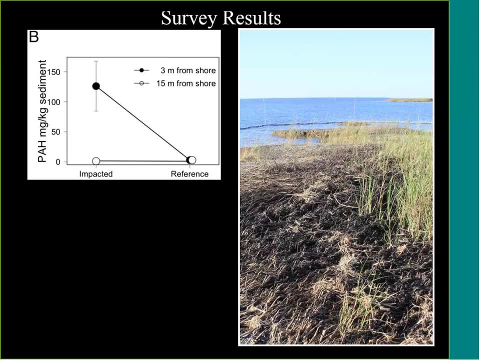 So there's another sort of service that these guys provided in this sort of anthropogenically extreme case. As I said, we also took soil samples and did chemical analyses on them, And so what I'm showing you here is just at 3 meters from the shore. 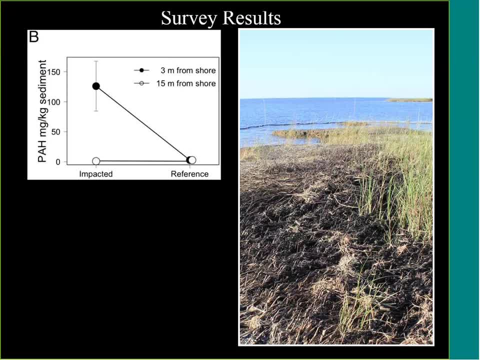 versus 15 meters of the shore, sort of based on this survey result: the concentrations of PAHs, again as an indicator of oil exposure, And we can see at the impacted sites. we see much higher concentrations of PAHs at 3 meters from shore. 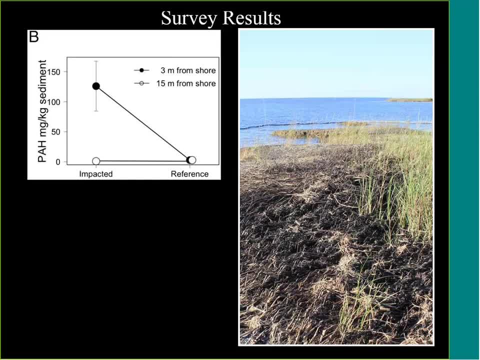 But over here in our reference we see that they return to references Back to the reverse. sorry, What we see is that at 15 meters from shore that we get the same amount of PAHs at the soil sites and the non-oil sites. 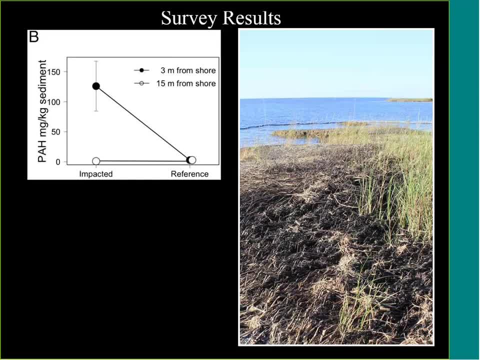 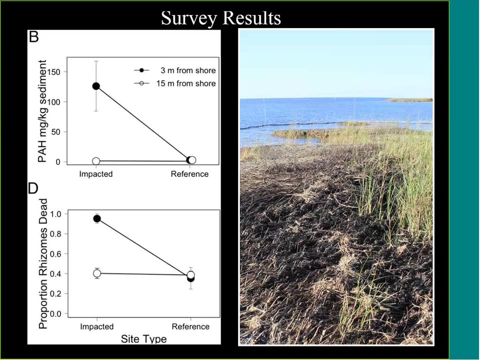 My legend there is incorrect, Whereas when we look At 3 meters we see that it's much higher. This legend should be down here And here we see. if we look again at the- Remember I mentioned that- that root matrix, the underground biomass and structure of these plants. 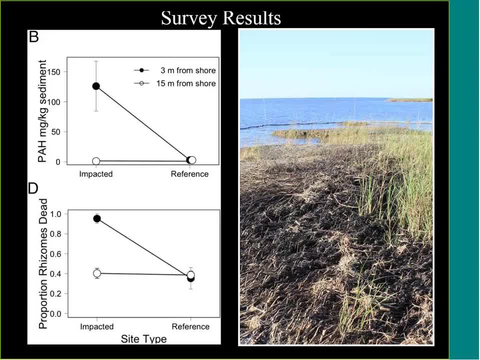 is actually the most important thing. We actually see the same kind of pattern with the number of rhizomes. The things that are required for that clonal growth and recovery are also really highly impacted. Almost all of them are being damaged and dead close to the water. 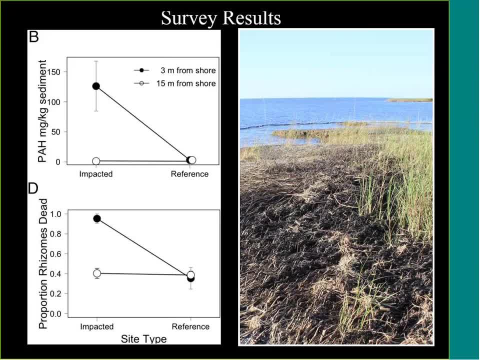 and most of them being, At least the proportion being dead, similar at the oil sites and reference sites when we move to our inland. So again we see this really concentrated impact close to the edge of the water versus So as we can see here, 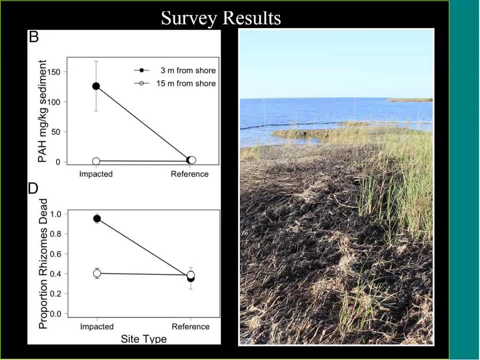 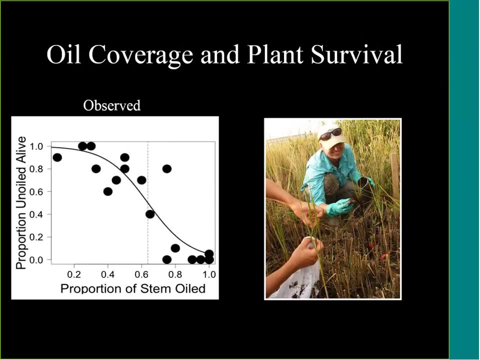 we're killing off both the above-ground and below-ground biomass in these cases, which we worry severely impacts and is different than what we see in those inland studies that showed that oiling kills the above-ground plant matter and not the below-ground. So just sort of to follow up on that a little bit more. 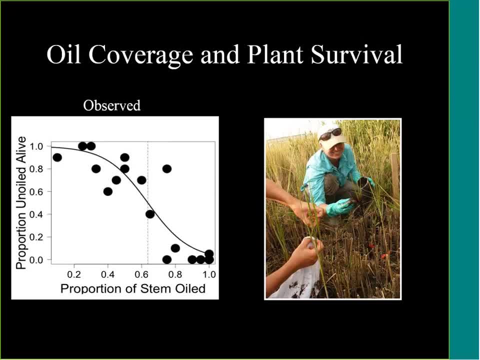 we also quantified the probability that the stem was alive. so what proportion of the grass was still alive, as a function of the amount of the stem that was oiled? So was it completely covered with oil, partially covered, et cetera? 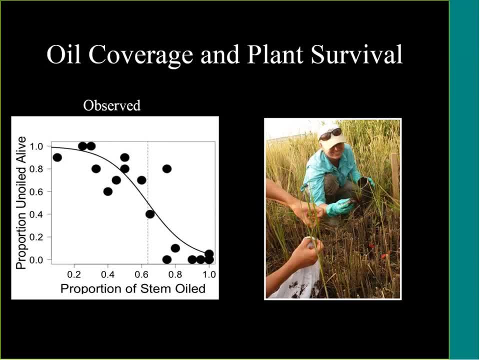 and did that impact the probability of the stem being able to survive and live through that stress? And you can see that there's a pretty interesting nonlinear relationship here. whereas as a proportion of stem, the stem that's oiled increases up to 100%. 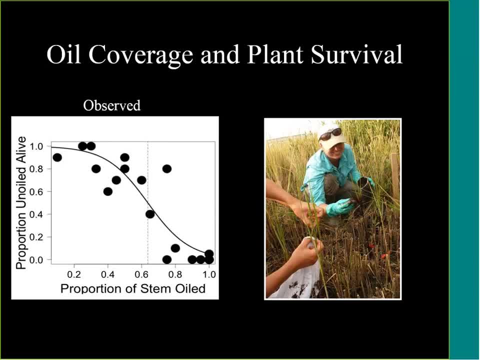 we see a rapid decrease in survival. In fact there's a threshold at around 65% oiling of the stem. So if the stem's covered by 65% of the stem is covered by oil, high mortality rate, You get sort of a rapid shift to death. 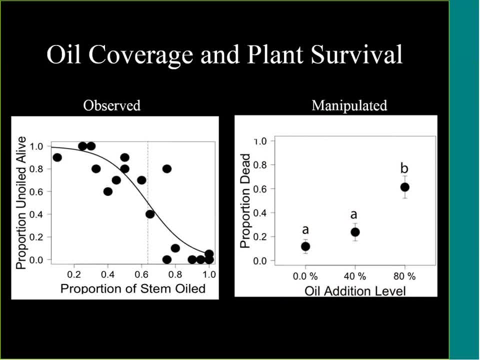 And we followed that up with an experimental manipulation where we covered the stem with either 40% of the stem covered with oil or 80% was done in a healthy non-oil place and we see the same pattern, whereas the percentage of the stem 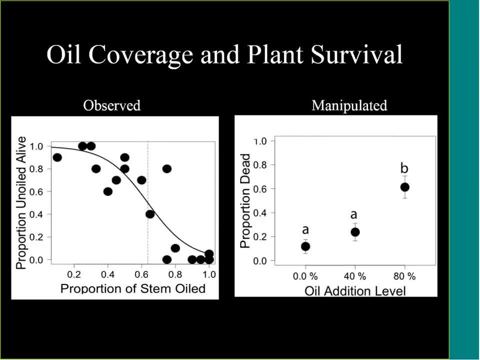 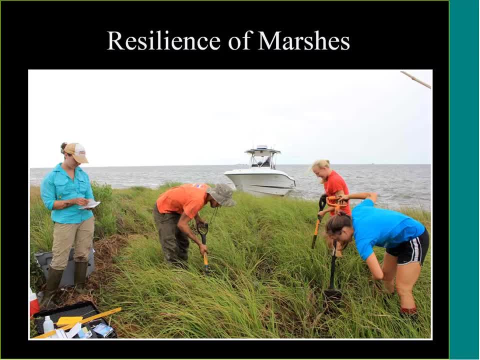 will increase. We see a high percentage of mortality of those stems. So we see that there's really severe impacts of this oiling event on the salt marshes, especially concentrated on the margin. But what happens to those marshes after the initial impact occurred? 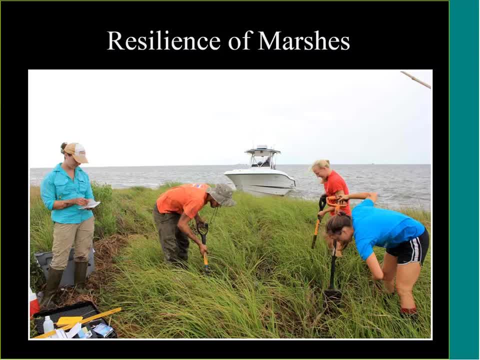 Did they actually respond in the way that we expected, based on those interior oiling studies, and regenerate rapidly, or do we see long-lasting effects of this oil, well beyond the impact of that oil? And so what we did is to determine this and most of the data I just showed you. 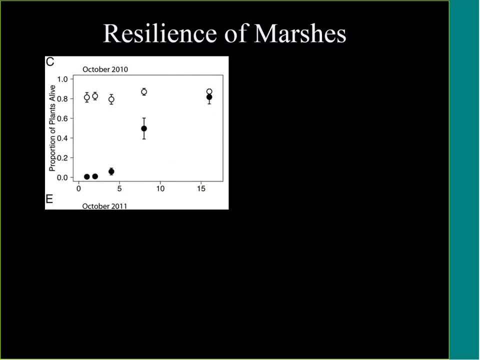 were five months after the oil spilled, approximately, And what I'm going to show you now is, from about five months post-spill to a year and a half post-spill, What we can see, what I'm showing you on these figures. 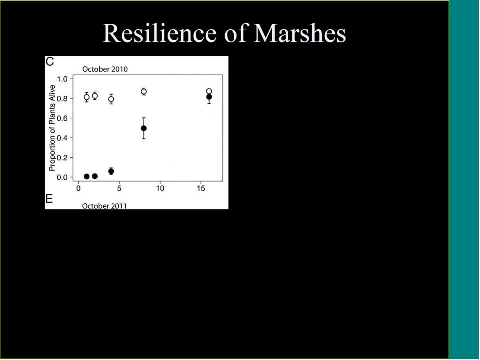 and this is again distance from the shoreline for our reference sites and for our oiled sites. this is the proportion of plants alive as we move along this. So this is very similar to what I showed you a moment ago as you move from near the water. 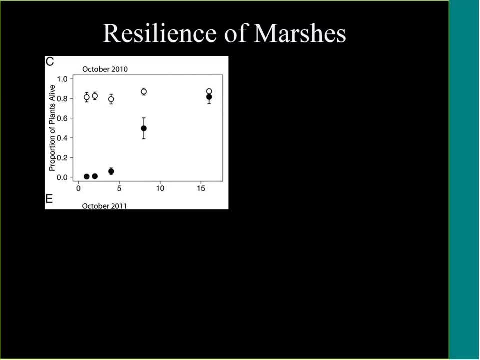 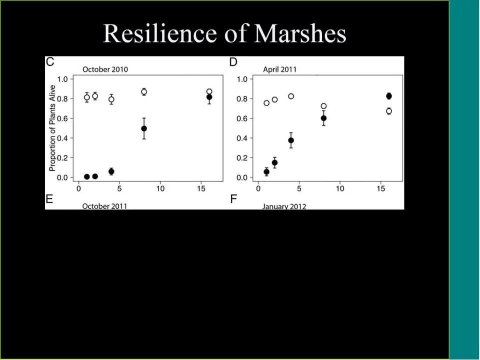 to far away, Far inland, a greater proportion of the plants remain alive. Most of the plants are alive in the reference location. So this is in October 2010.. We go to April 2011, and we start to see that at this intermediate distances from the shoreline, 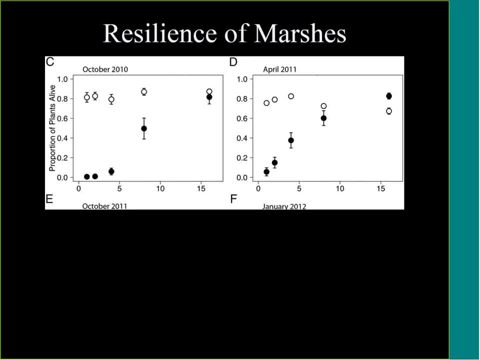 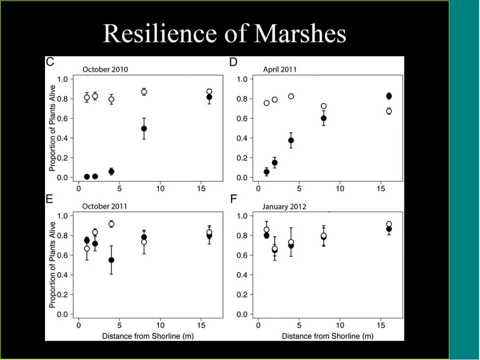 we start to see the impact of sites looking more like the reference sites, but we still see a high proportion of plants dead near the shoreline. However, as we go into October 2011 and again to January 2012,, we see that actually the proportion of plants alive. 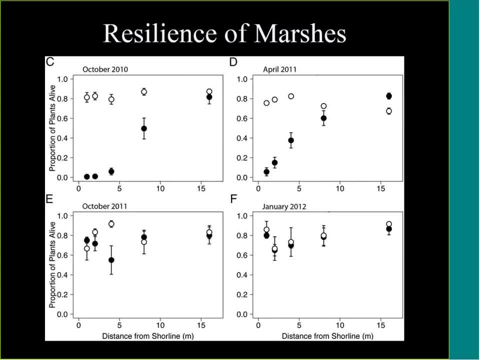 actually converges on the reference sites. We see this really encouraging result that these salt marshes have recovered quite well and actually mimic those reference sites that weren't impacted by oil, So this is a really optimistic thing. This isn't that long after this really devastating impact. 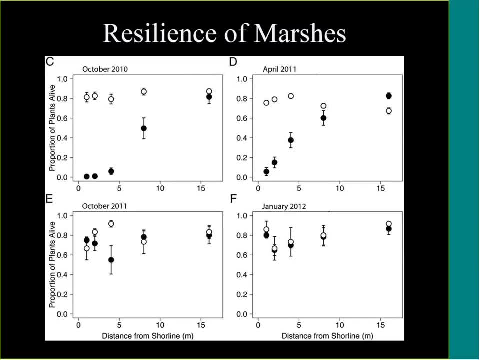 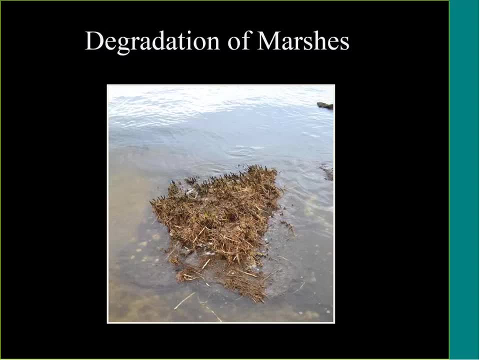 to see this kind of recovery of these salt marsh plants all the way back to a reference level. However, it's not all optimism in this case, and that's because, like I talked about in the beginning, these salt marshes are already highly degraded. 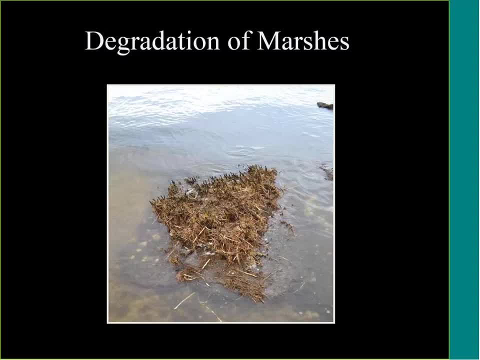 And so, in addition to losing those grasses, we have conditions set up where huge chunks of the edge of the salt marsh are being broken off by wave action, because they've already been degraded to a point where they no longer have their natural, gently sloping edges. 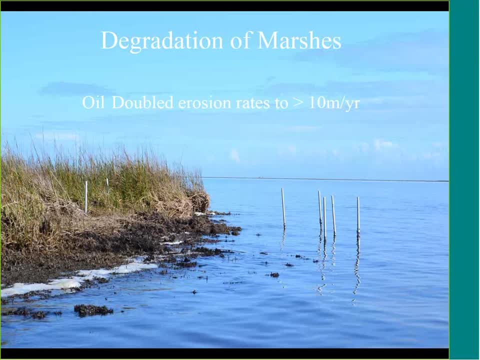 And so what we actually found? despite the rapid recovery and resilience of these salt marshes to the oiling effects, we see that the oil doubled the erosion rate by more than 10 meters per year, at least during the time period until the salt marsh grass is recovered. 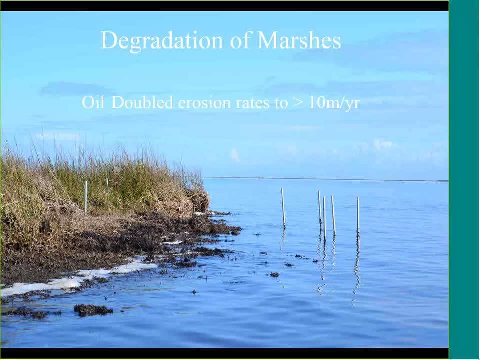 So over that year and a half time period in some locations we lost 10 meters of salt marshes. That's a lot of area loss. That's a lot of area when you spread that across potentially 75 linear kilometers of shoreline in Louisiana. 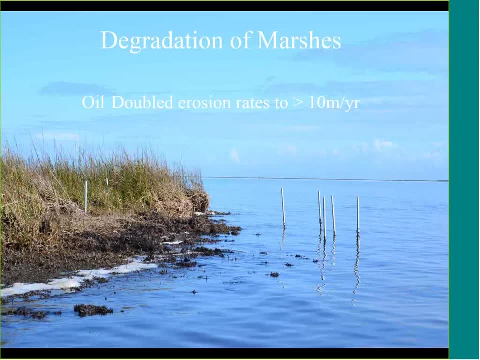 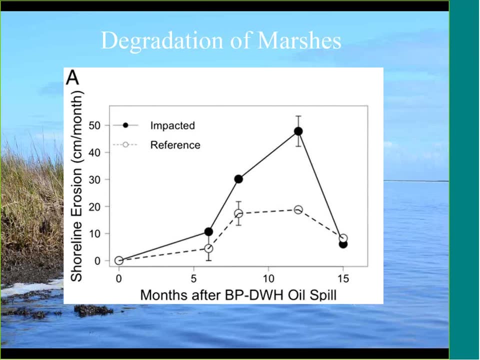 That's a lot of landmass being lost. Not that every location lost that amount, but So, in fact, look at months after the oil spill. we look at the shoreline erosion rates. We can see that at the Just as we saw with the grass growth. 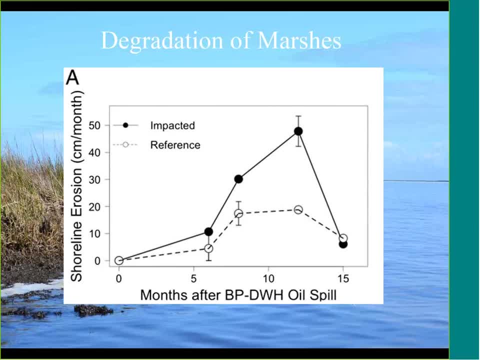 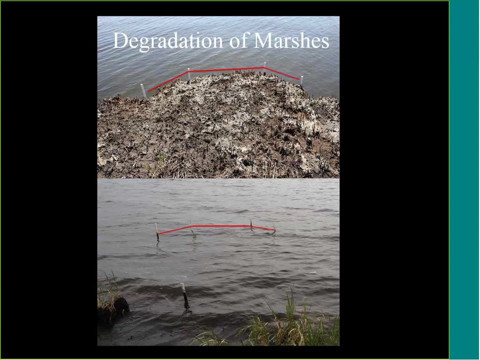 we can see that the erosion rate. Actually we turned around 15 months after the event actually occurred. but the problem of that is is during this region, when we weren't returning back to those pre-spill erosion rates, we lost a tremendous amount of salt marsh area. 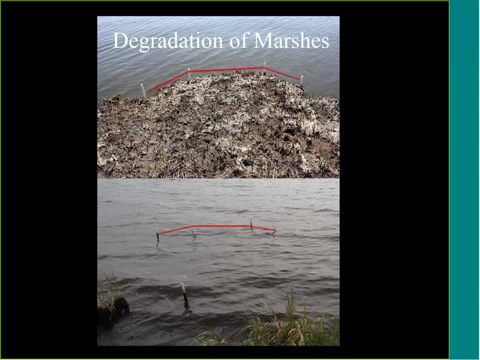 And so here you can see an example of that. I just added this red line here to outline the edge of the salt marsh at the beginning of the survey, and here are those same pipes 15 months later. So we can see that, although the grass 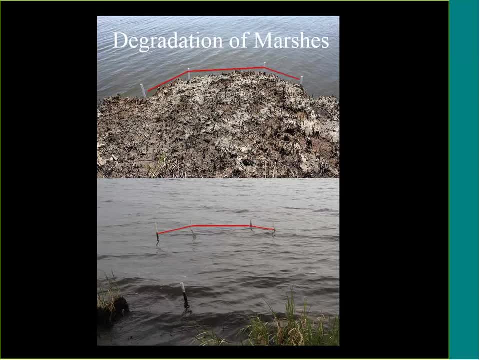 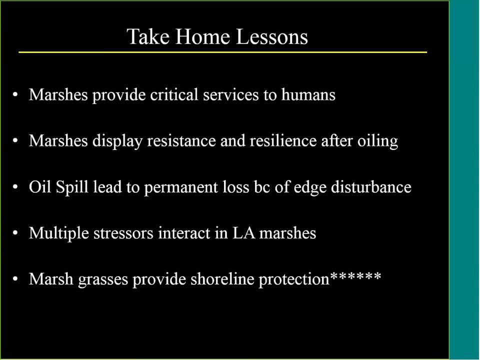 into this area. they can't recover into areas where the marsh no longer exists, So we still have this massive impact to deal with. So what are the take-home lessons from our work? First, I think it's important to recognize and to inform people. 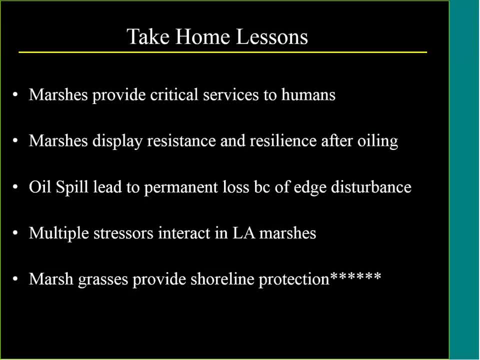 that these marshes provide really critical services to humans, and in fact, much of the coastal economy is dependent upon these marshes, and I'm not sure that many people who live in the coast actually are aware of that. These systems display remarkable resistance. 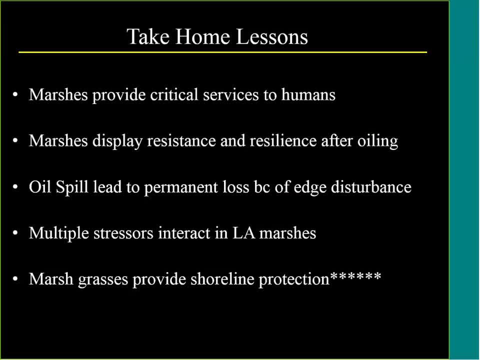 and resilience after both natural disasters as well as sort of more anthropogenic disasters like whoa oiling. but that resilience is not in itself going to save these systems because, as we saw in this study, the oil spill led to permanent loss. 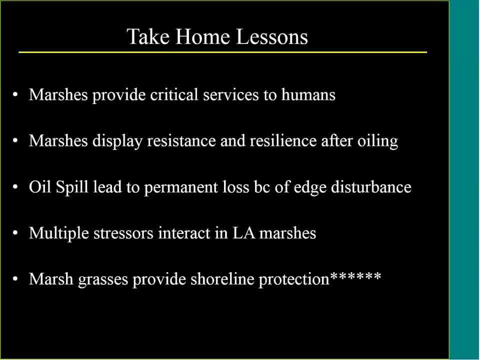 of the edge of the marsh because of erosion. So, despite the resilience of these systems, once you remove it you can't recover it. It's really hard for these systems to recover once that land mass has actually been involved, Sort of a subcomponent of that. 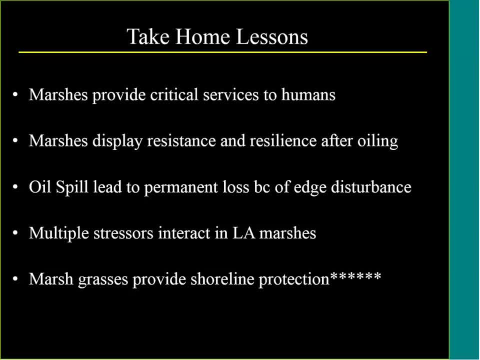 that we didn't measure, but I think is really important. I talked about these systems as carbon sinks. Well, as that shoreline is taken away and that carbon is re-suspended into the water column, it's eventually going to end up back in the atmosphere. 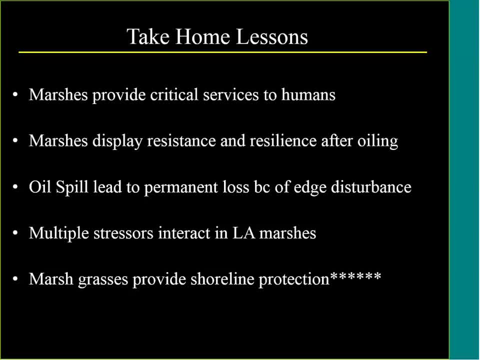 so it's also releasing a bound of carbon back into the food. well, So that's a really important thing to think about. And then, as we go through this, we're going to talk about the environmental impact of these systems. So we're going to talk about. 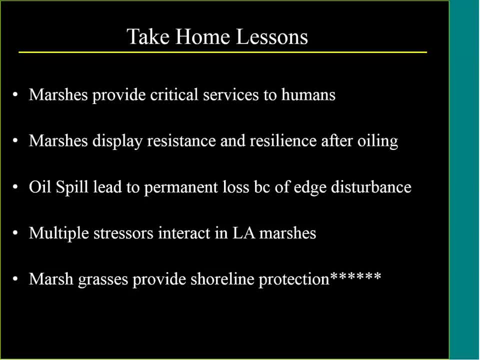 the environmental impact of these systems and how they're going to contribute to global warming gases. Also, a take-home message is that multiple stressors interact to affect both how natural disasters will impact these systems, but also how they can respond to them. So 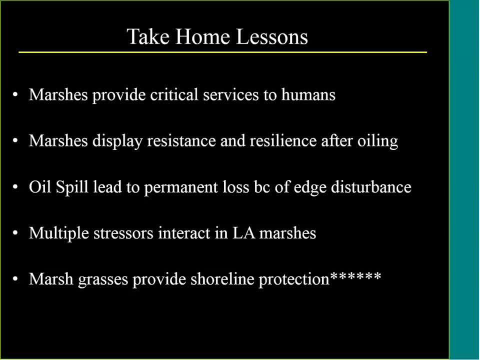 you can't just think about the ecology of the systems without also thinking about the history of what they've already experienced, trying to evaluate how they're going to respond to these kinds of disasters. And the most important thing is that these marsh grasses provide shoreline protection. 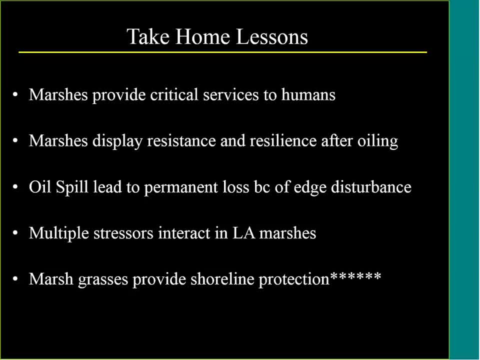 They provide shoreline protection, in this case against oil moving inland. They actually concentrate it right at the edge, which minimizes impact potentially, but also provides protection against other kinds of coastal events, hurricanes and so forth. So with that, 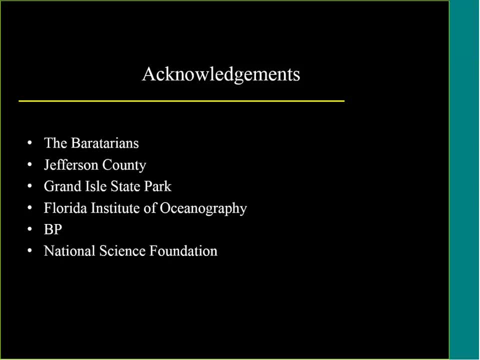 I'd like to acknowledge a variety of folks who helped fund or give us access to the area to do this work, and I'll be happy to answer questions if anyone has any. I know this wasn't your aspect of the study, but you mentioned. 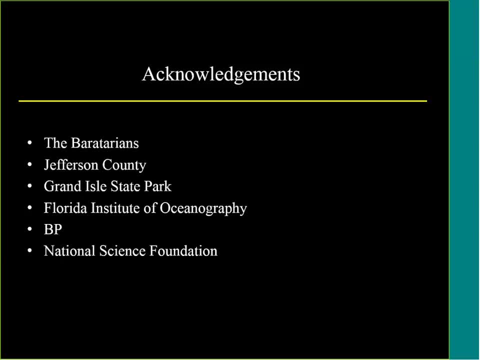 that people looked at the associated animals in the marsh and I was wondering if anybody, if you, just in a nutshell, if you could say anything about the general trend as far as grazers: maybe reduced pressure, or did grazers come back? 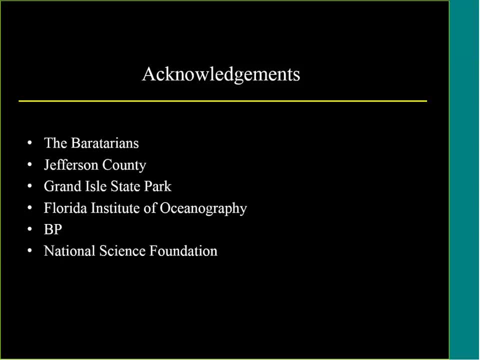 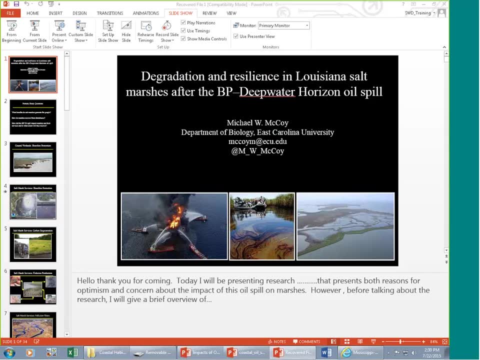 with the marshes as they recovered and things like that. I anticipated that question. That's why, Oh, it's not on the one that I gave you. Oh, I just did it a minute ago, which is good, Okay, So. 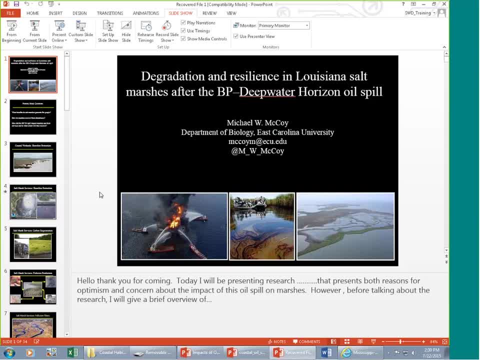 anyway, what we did find is we saw reductions in the numbers of crabs, reductions in the number of mussels and reductions also in the number of periwinkles, Unfortunately. so the numbers of the periwinkle snails in particular. 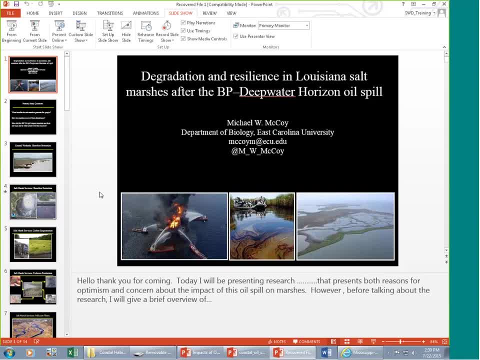 were already low across all these sites, and so we didn't see a huge difference in survival from those. We saw significant effects on both fiddler crabs and lead crab abundances, and also on the periwinkle snails as well. 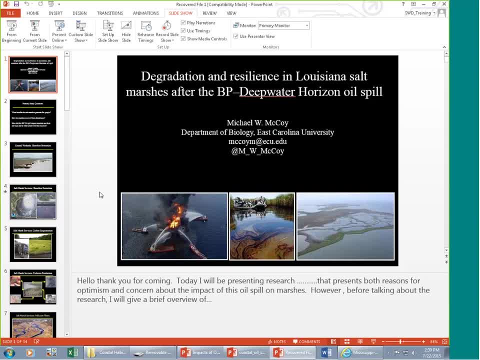 So we did find that there was a significant increase in survival on mussels. However, we were hesitant about incorporating or saying too much about their making big differences, because that was sort of incidental data we collected while doing the other surveys. It wasn't a target. 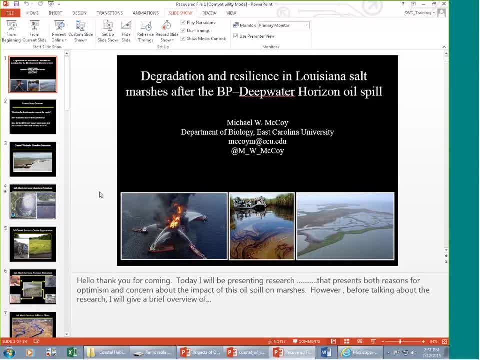 of the study. so we didn't actually dig up the burrows. So of course we did some burrow counts. We did surface counts, So it's not super rigorous, but the trends that we found were no different, Very same. 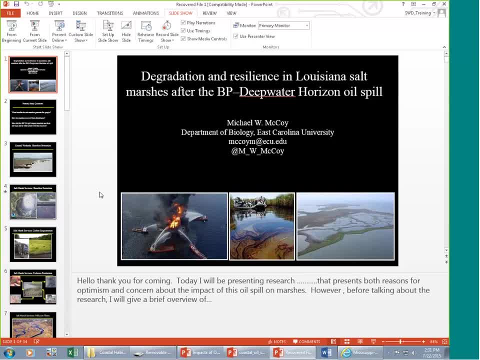 patterns we saw with the crabs, Just not quite as more variable and not quite as significant. I just at the last Gomery conference there were some presentations that also discussed the ants and the study that was conducted on the ants showing there. 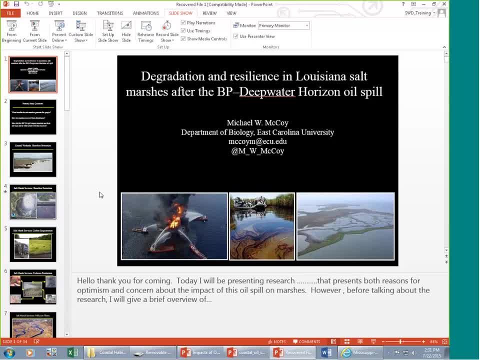 was significant impact to the ants that were living in the soil. I don't know what the fact of that citation was, but it was an interesting presentation. They showed some significant impacts. I'm not surprised at anything, since you know, just thinking. 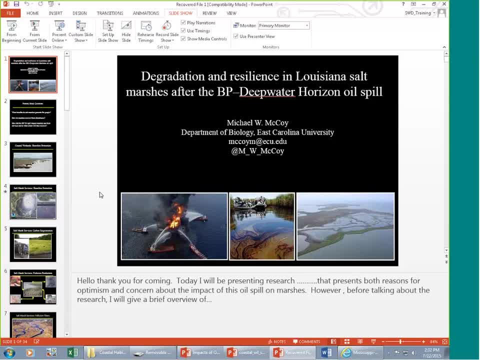 about the fact that the oil caused massive death of the sort of root matrix which is what things like mussels and fizzler crabs depend on to be able to survive in the soil. I don't know that particular study, but I would imagine many. 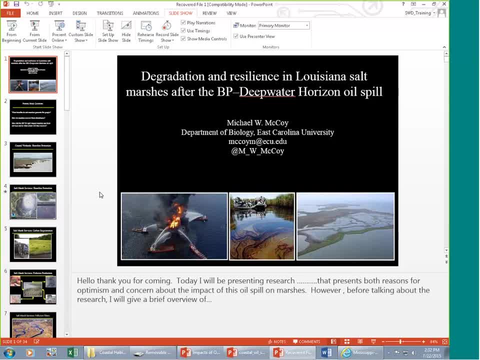 things, especially in all the waiting for the feed on. this creature probably also would just like to feed along the edge of the soil. It's very interesting, I enjoyed it. You said you didn't have to post Rita and Katrina, so we got. 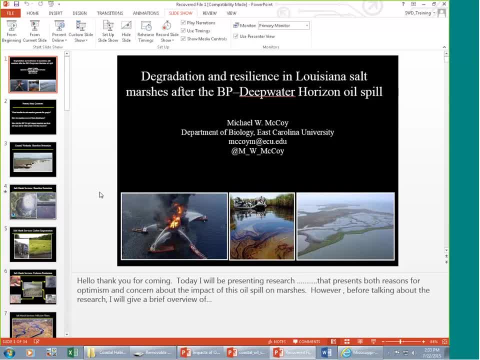 seedlings everywhere. They were true seedlings. Yeah, I know, and often that is the case, that seed dispersal is a really good source. I don't remember I wasn't a part of the study that I was going to hear. that was. 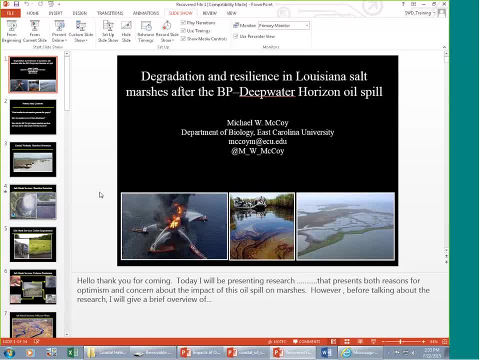 actually Dr. I don't remember what the name of the seed was, but it's encouraging to get massive seed. in addition to genetic diversity, Did you find that the die off of the farm finder was that mostly from blocking photosynthesis because it covered? 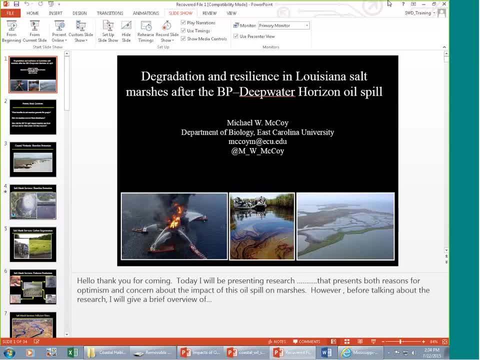 those leaves, but also from toxicity, and I think the root dial was called- by the high pH concentrations. I don't know that for sure. Most of your report talks about plants, so what I have not, I know, Dr Schillingman. 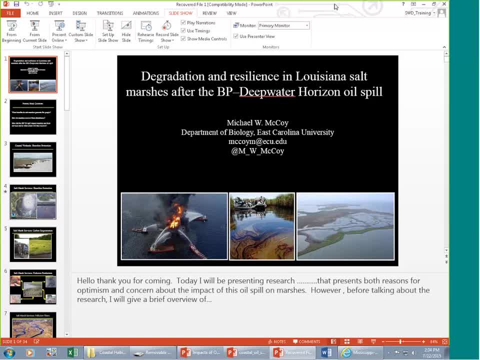 has ongoing work in the system. One thing I have looked at is the erosion rates. although they close to reference levels, have actually continued at a slightly higher rate. I think that there is a lot of work. 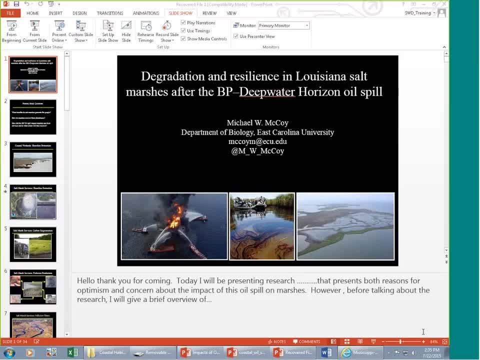 but there was. there was definitely some variation place to say, but it wasn't. 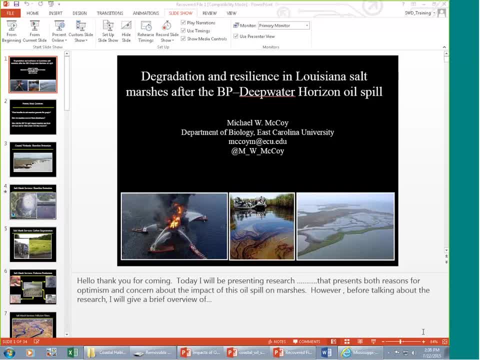 like near, near reference to really extreme. they were all sort of at intermediate whaling levels and you can see that in the sort of confidence intervals on the pH figures. were all those sites free of like any cleanup techniques applied to them or was it just, you know, it got oiled over and was? 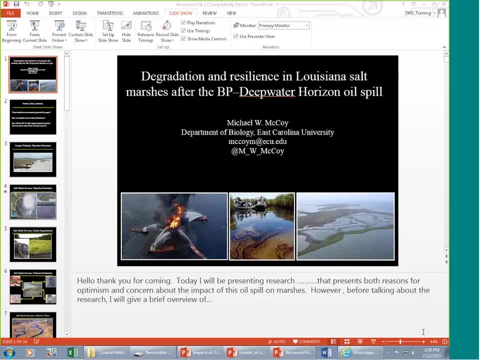 kind of left for. yes, so these particular sites- they were near sites, meaning and some of the spraying superheated water and stuff, but not these direct sites were affected by that. I think dr Silliman had some simultaneous work going in and sites that were treated versus not treated out, so there's a 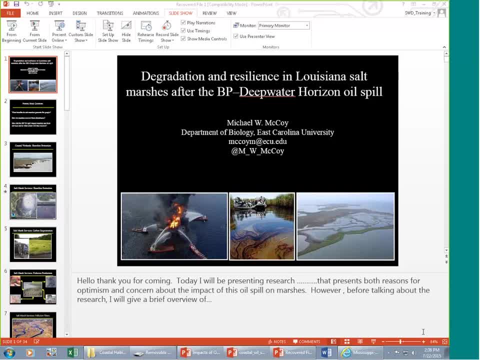 question online about if you notice any damage from booze in operation. do they have any um um? so in some of the sites they did put booms after the initial oiling event just offshore, and there I don't know of any direct damage that I can point to.